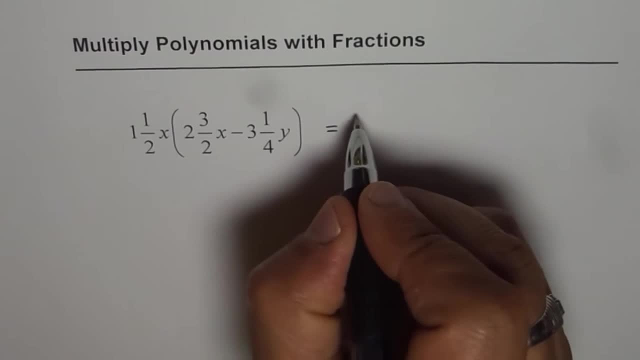 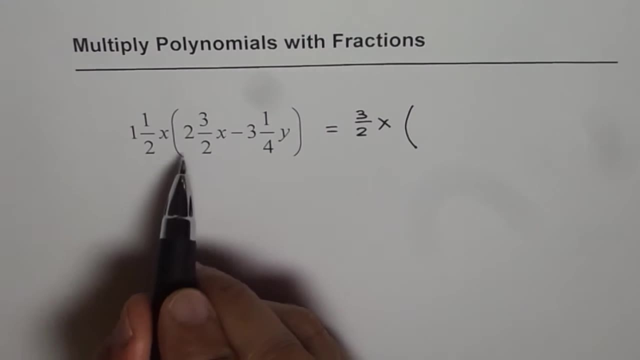 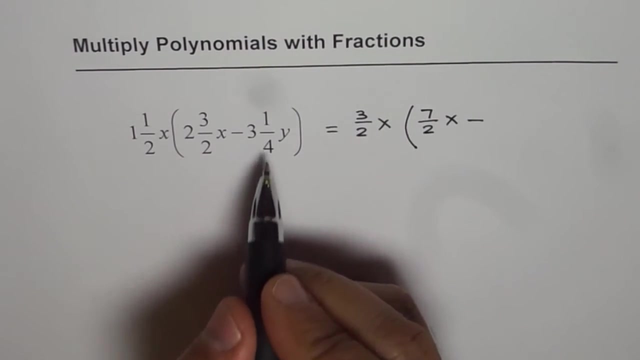 written as: 1 times 2 is 2, 2 plus 1 is 3, as 3 over 2, right, So we have x here. times 2, 3 over 2 can be written as: 2 times 2 is 4, 4 plus 3 is 7, 7 over 2x minus 3, 1 over 4, 3 times 4 is 12. 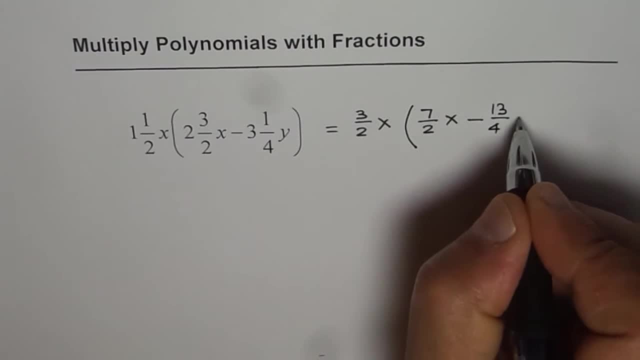 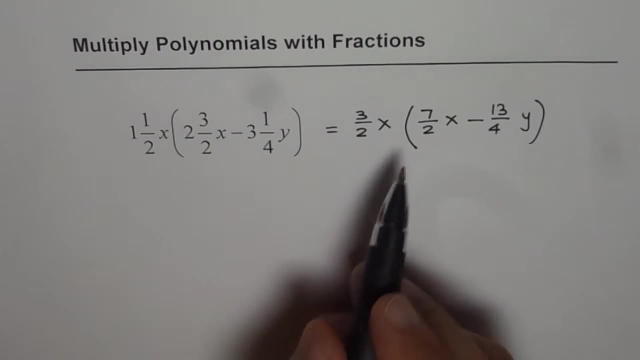 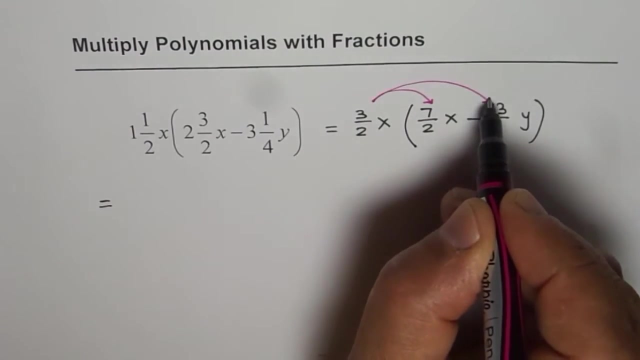 plus 1 is 13,, 13 over 5y. So that is the first step. So first step is to convert improper fractions to, I mean mixed numbers to improper fraction. Now the next step is apply the distributive property, That is to say that you multiply this term with both the terms inside. So let's do that. 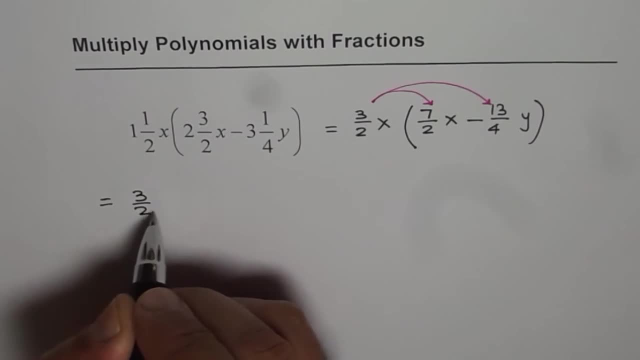 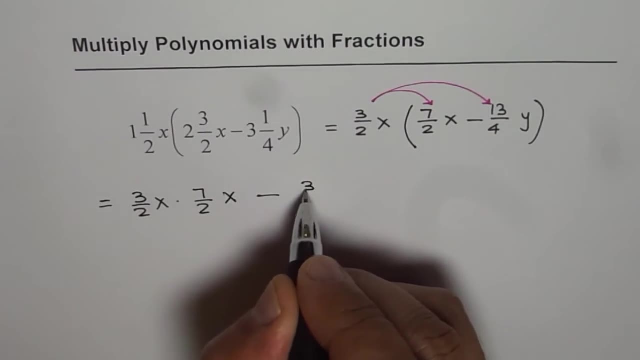 part. So it is 3 over 2x times 7 over 2x minus 3 over 2x times 7 over 3y. So it is 2 plus 1 over 3y times 2 times 3 over 2y minus 3 times 7 over 2x times 7 over 2x. 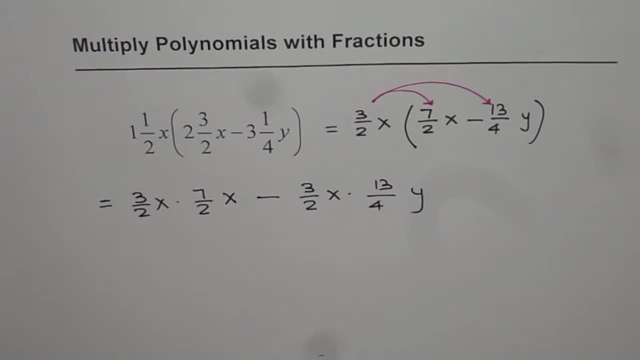 加 4 over 2x times 7, plus 5 over 3y times 7 over 2x. Now this minus 3d is going to be equal to 13 over 4y. so that is by distributive property.